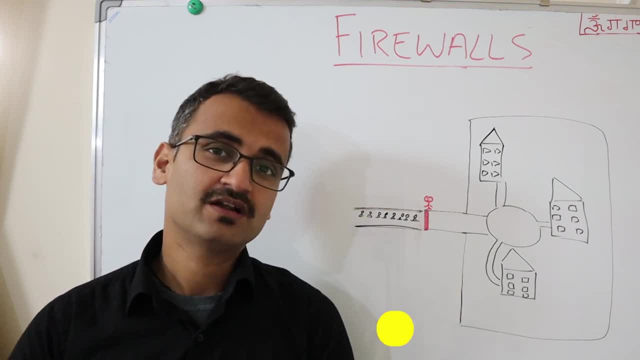 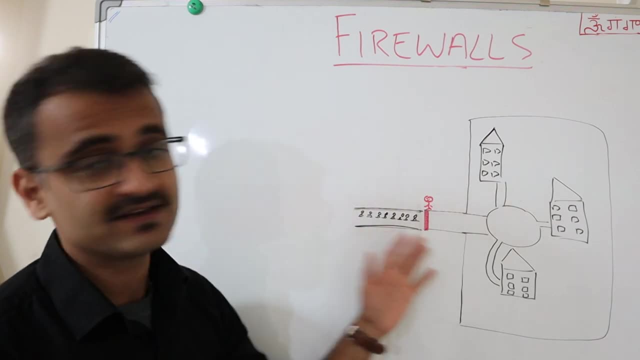 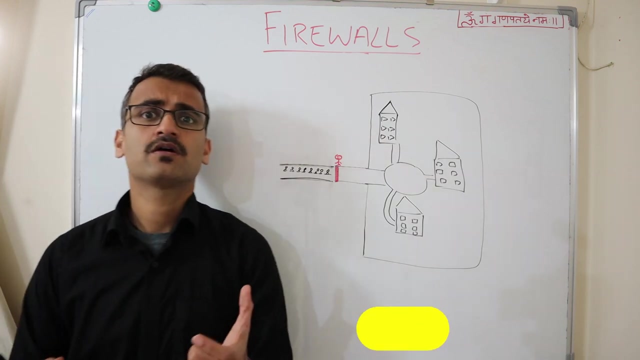 firewall, the security guard, ensures that only the legitimate and the valid, uh you know users or guests or visitors uh enters the society. so firewall is nothing but a security guard. firewall which is a sort of a conscious router as well. you can say uh, which enables you know that only the 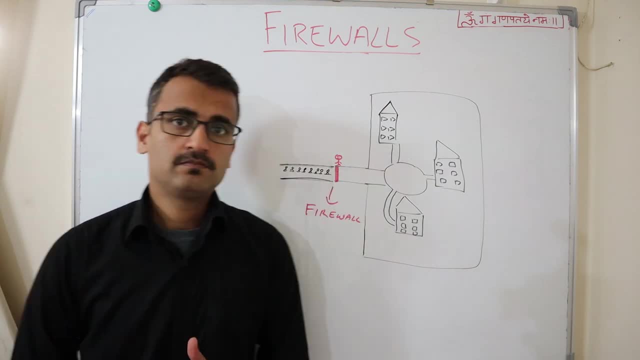 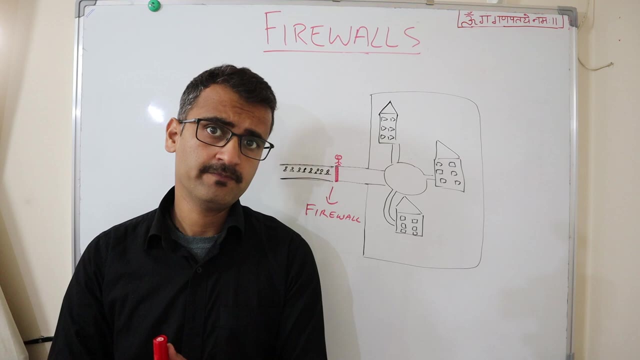 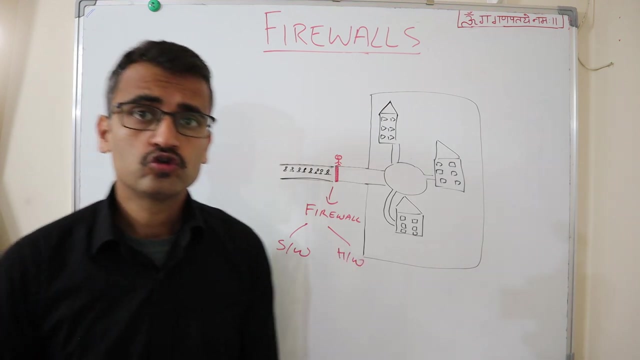 legitimate network traffic gets into uh, the you know the network. so, friends, uh, let's quickly discuss about the two main categories under which a firewall, uh can be divided. so the those two categories are software firewall and hardware firewall. so hardware firewalls are actually the hardware appliances which you put in the perimeter in your network to be able to connect to the network. 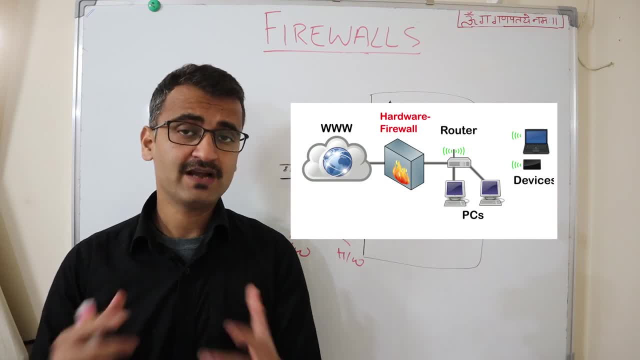 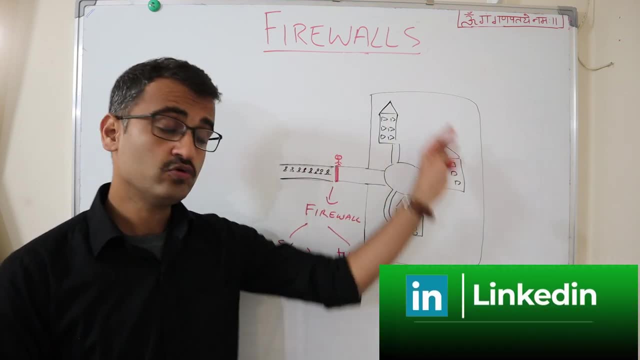 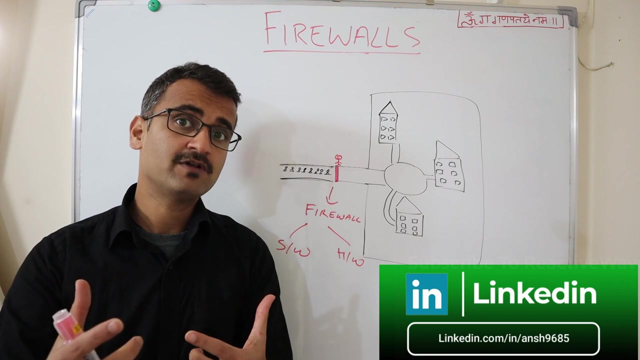 boundaries so that no intrusion can happen, and that particular hardware firewall can be equated with the security gate and the security personnel who's, you know who's- securing your whole society. but a software firewall is also, you know, an operating system level firewall which is installed in on your specific systems. like you see, windows firewall is a very good example. 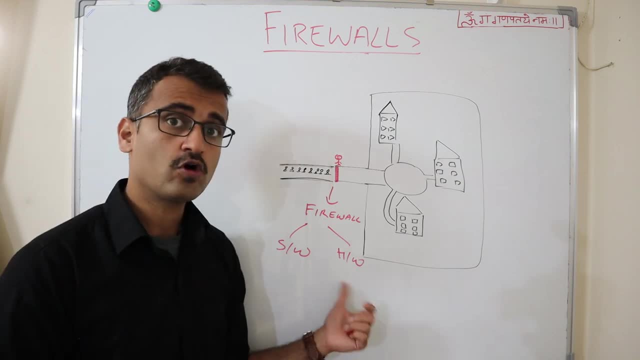 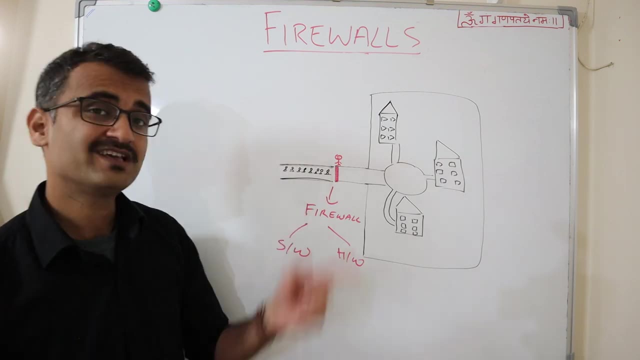 now the question arises whether we need a hardware firewall or a software firewall. so you should ideally be using both. why it's very natural? because, suppose this security guard is a very good guard and the gate is very, you know, very- strong gate. still, if you are staying somewhere, 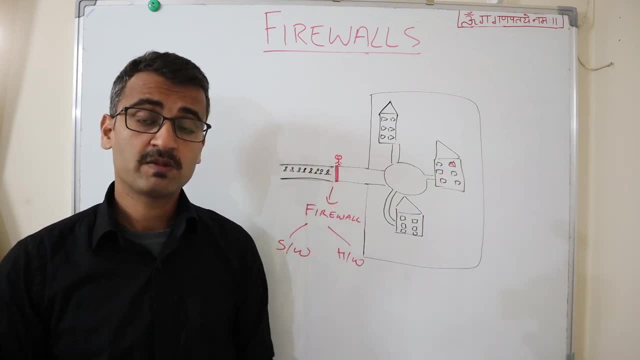 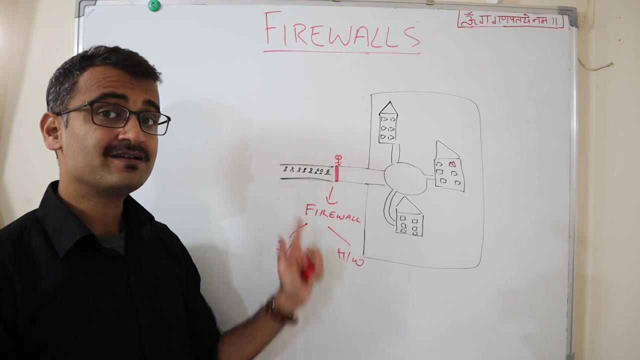 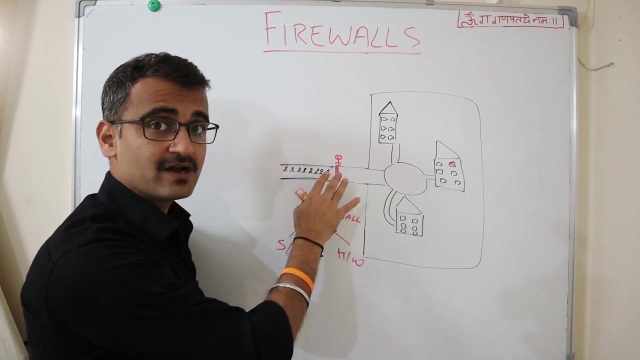 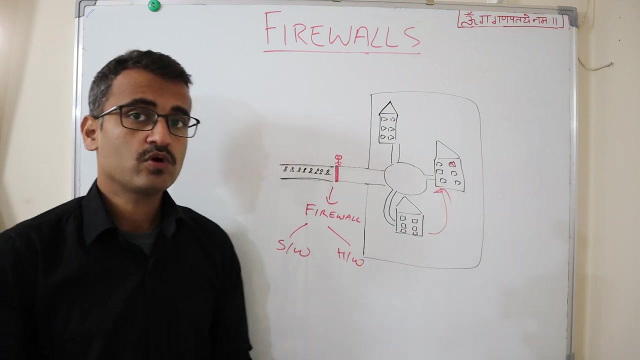 here. uh, you still would put a lock in your house to give that additional level of security to your house, because the intrusion might not be external, it could also be internal and your firewall guy is sitting only securing the outside traffic coming into the you know the your network. but what about if some intrusion happens from here to here? then what? 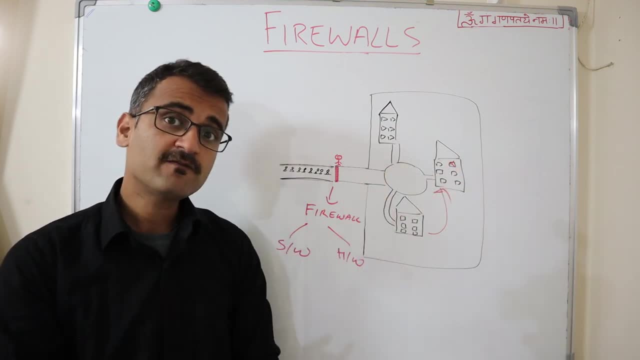 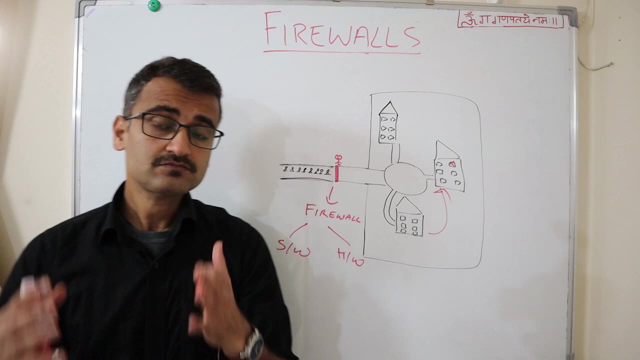 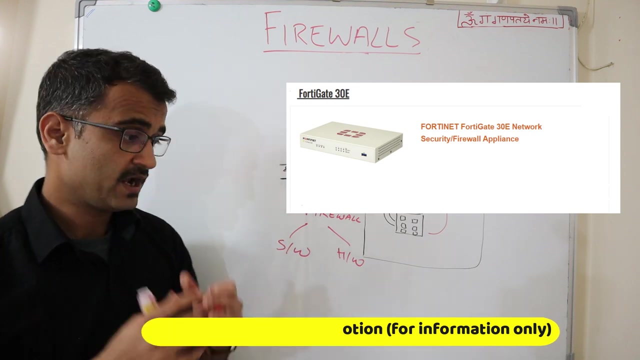 would happen if something happens within the society. so your software firewall acts as a second layer of protection. so always understand this difference between the two. also, your hardware firewall can be a standalone appliance which you know, which can be deployed. uh, only looking and making sure that you know it is acting as a dedicated firewall, or else, or most of the route. 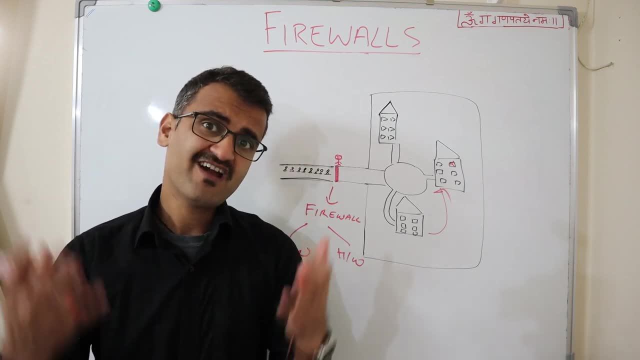 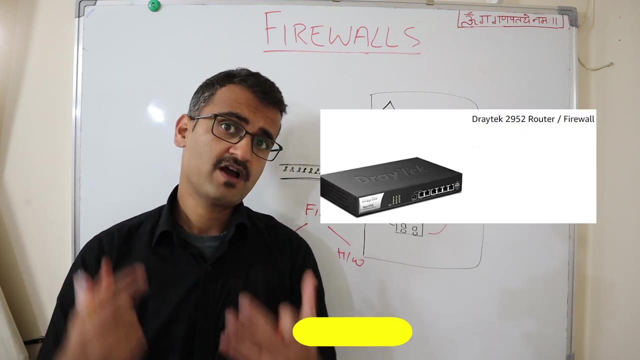 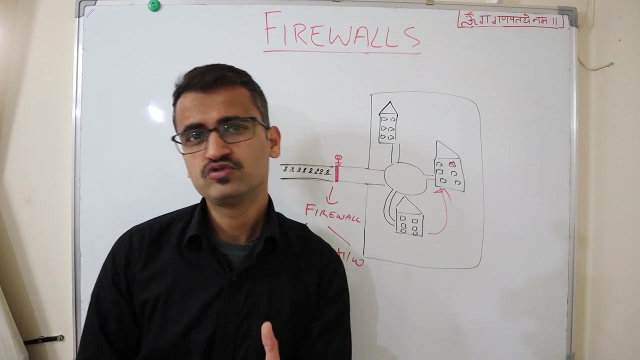 are also now coming up with the firewall functionality, so you can have both a router and a firewall. so a router's responsibility is to route the traffic to the- you know- correct direction, wherein the firewall would ensure that only the legitimate traffic is passing through that router. so a small great company or a small usage scenario might take both into one device: router plus. 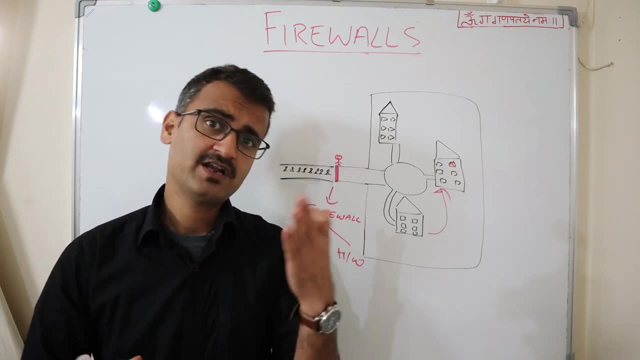 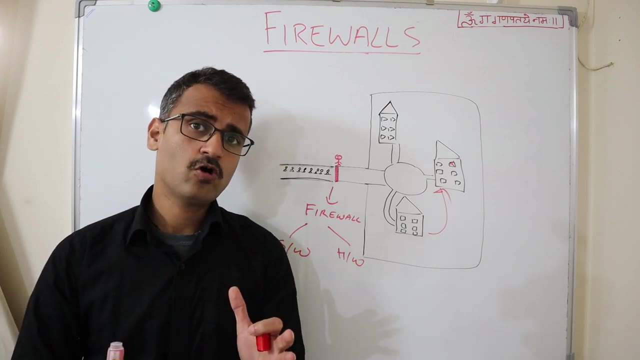 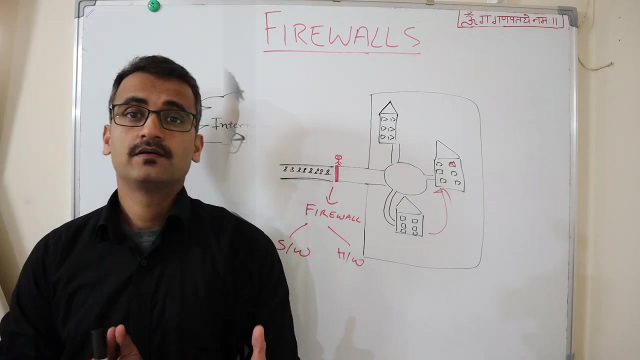 firewall, but maybe at an enterprise level you might have a dedicated firewall device and a dedicated router. so it depends. so, yes, so this is the basic understanding of firewall and the two broader categories. now we'll dig deep into the basic architecture of how firewall is designed. so, friends, this is. 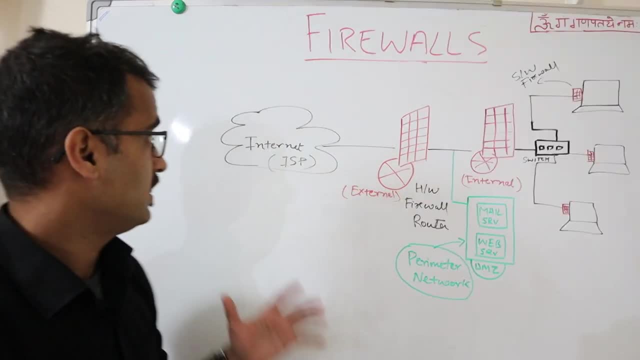 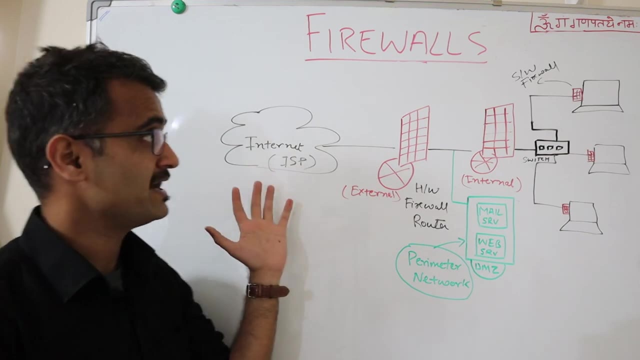 a high level architecture of a firewall design. uh, so, as you can see from on the left, the traffic is coming from your internet service provider. this is your extranet, your external network, and then, uh, you know, these are the two firewalls which we have placed. this is the external firewall. 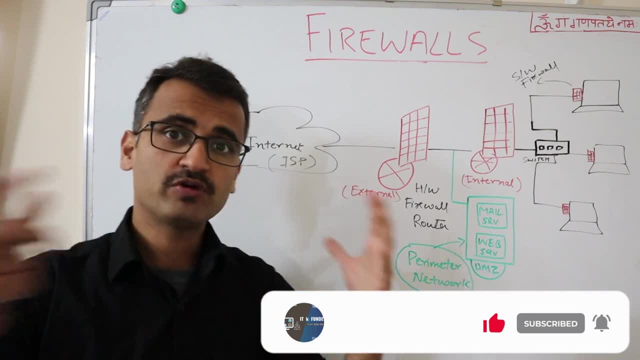 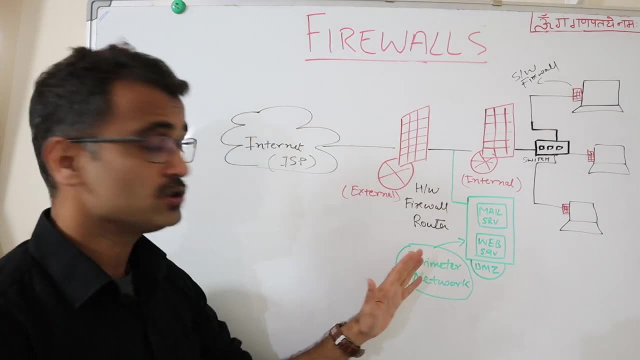 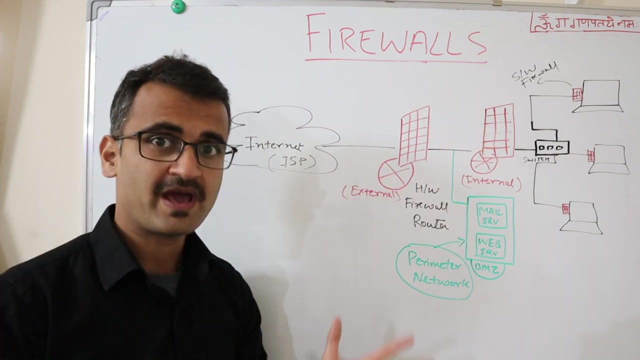 and this is the internal firewall. you you know you can design your architecture with a single firewall also, but this is to just give you that additional layer of security. and also the benefit of this is that if you have an external firewall and an internal firewall in between, you could have your parameter network. 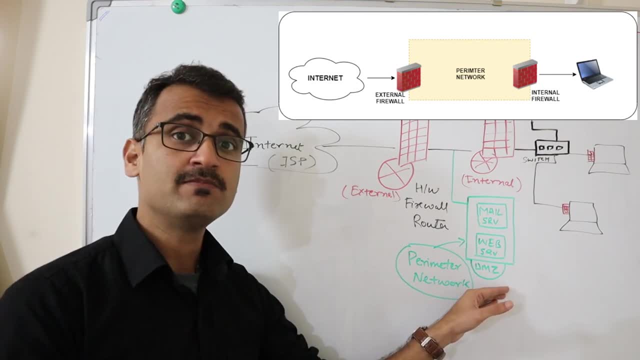 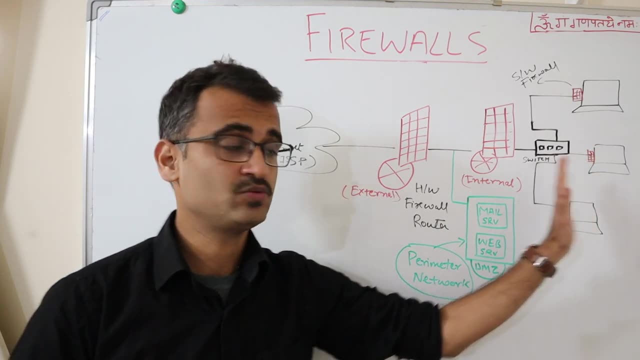 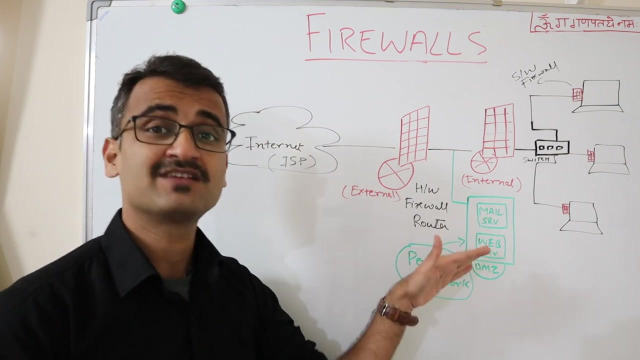 in which you can host your dmz, which is demilitarized zone. now, what is a demilitarized zone? this is an area which is lesser restricted than your actual local area network in this area. so the application is a dmz and this is a dmz function which is designed to be used in 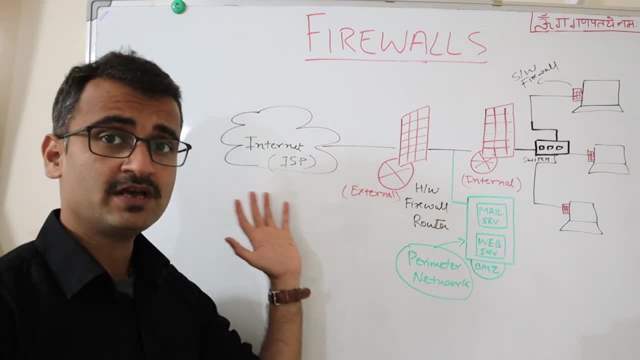 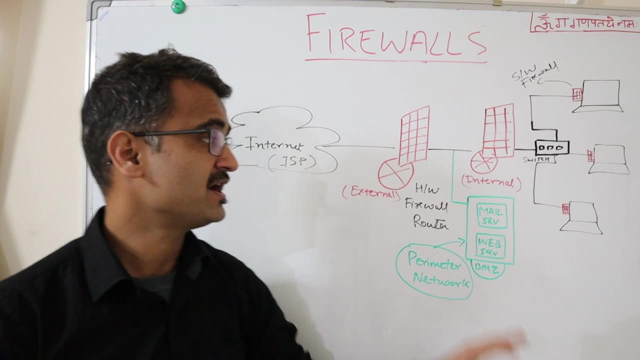 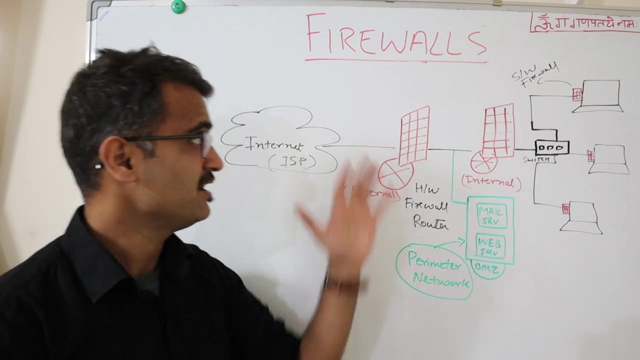 the network for your web servers or the applications which needs lesser restrictions, like your mail server. anyone on the internet might want to connect to your mail server. anyone in the internet might want to connect to your web server with lesser restrictions. so instead of placing it within your local area network, you place it into dmz. so dmz is also a functionality. 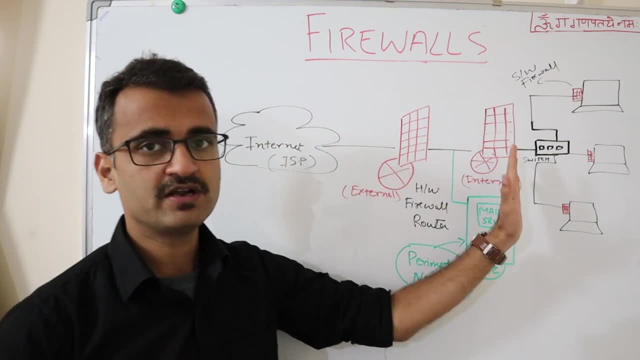 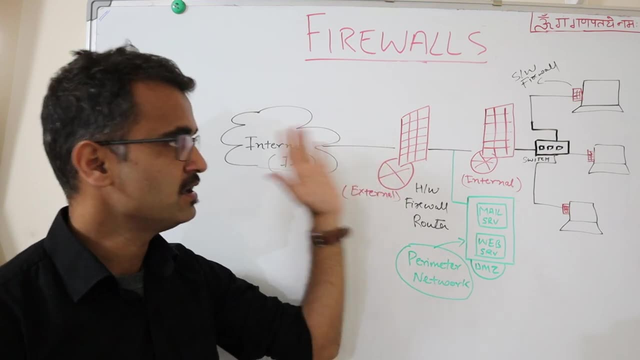 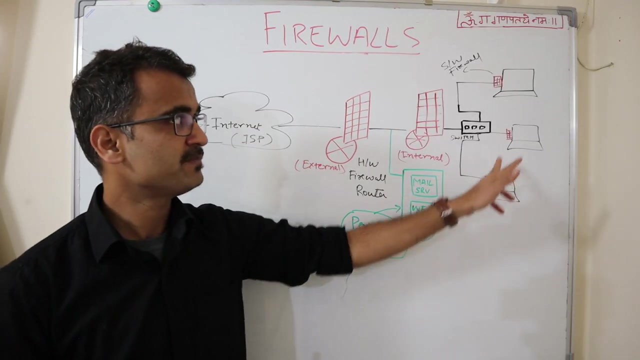 which is, uh, you know, designed using a firewall parameter, uh, perimeter network firewall, the, you know, any request which comes goes through the rules which have been set up and based on that, the decision is made whether this should go ahead or this should go into trash. and then you have specific software firewalls which are deployed in every machine at an. 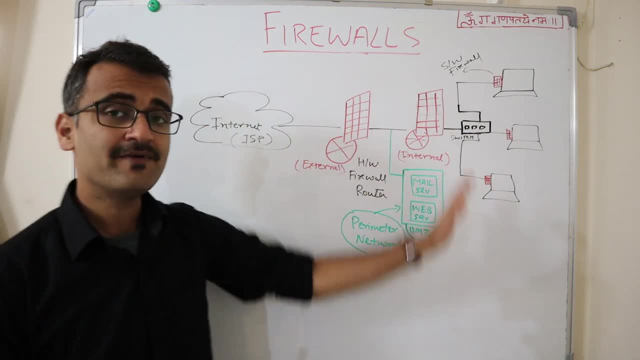 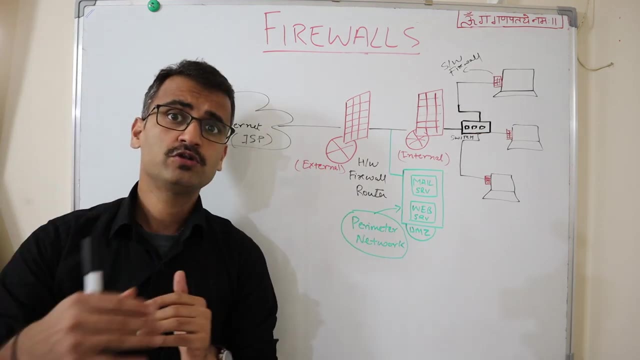 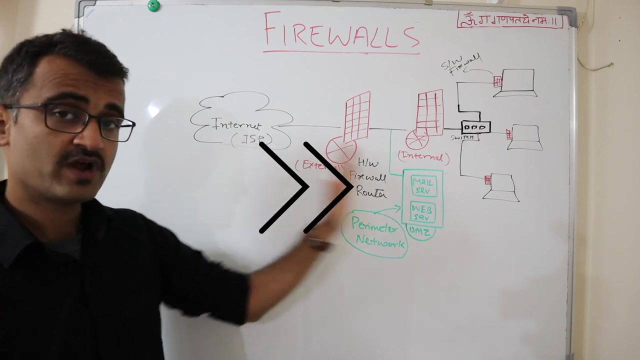 operating system level. so, yeah, this is a you know an overall architecture of a firewall and then always understand that there is a priority in which you know the rules are set. so anything which is going from left to right in this diagram, so what is in your left, left is external and right. 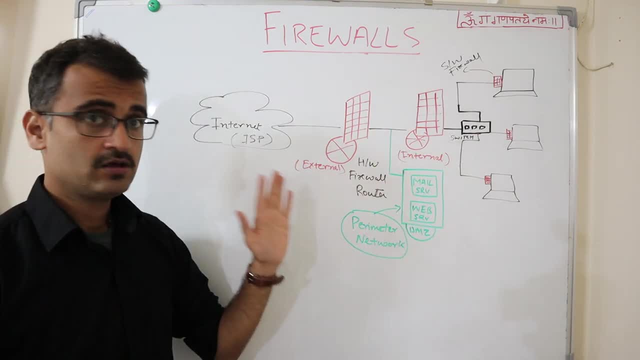 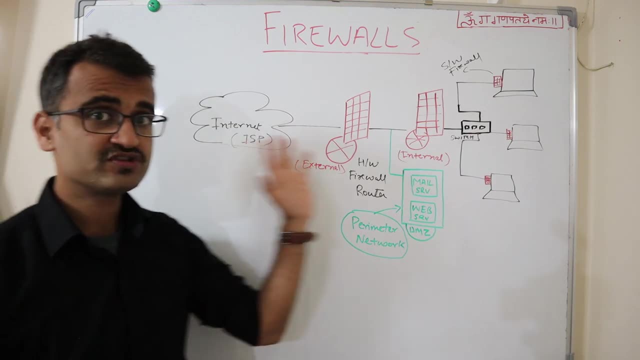 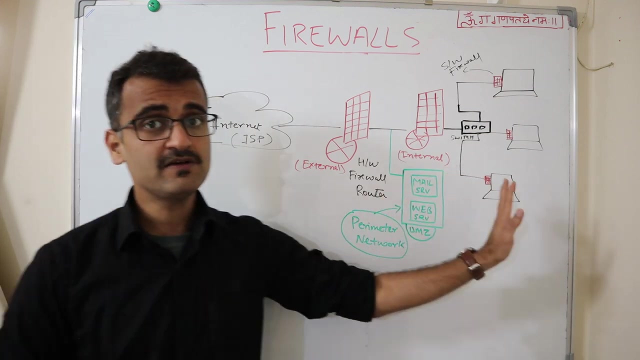 is internal. okay, so from left to right you have lower priority. what does that mean? that these would be more restricted. anything coming from outside to inside your network would be more regressively tested. okay, wherein anything coming from you know this right side of your local area network. 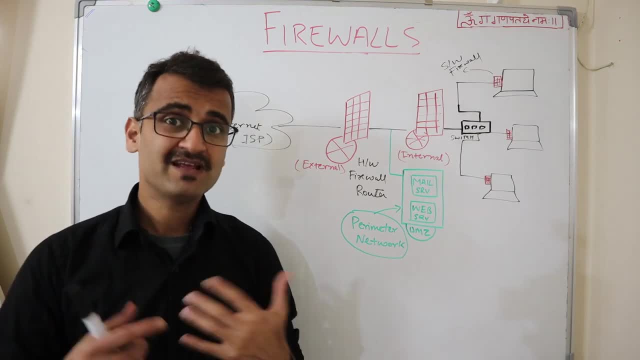 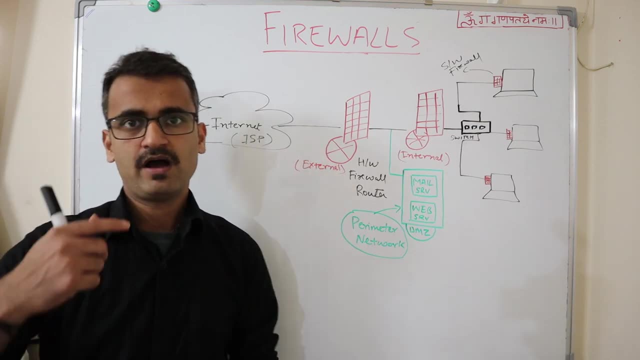 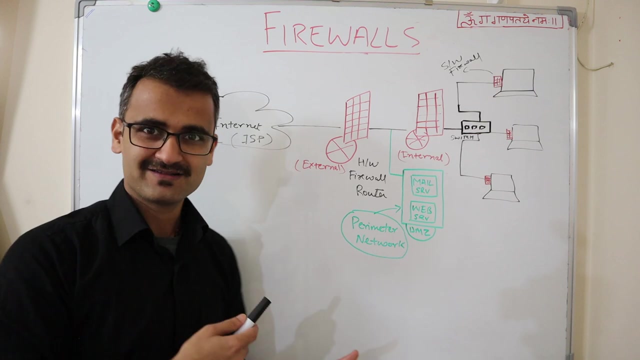 towards outer network would be, you know, lesser restricted because this has a higher priority. so take, for example, if we take our society, a visitor entering into the society would be grilled more by the security guard, whereas an owner, if he is walking past the security entrance gate for a morning walk, maybe outside the society, 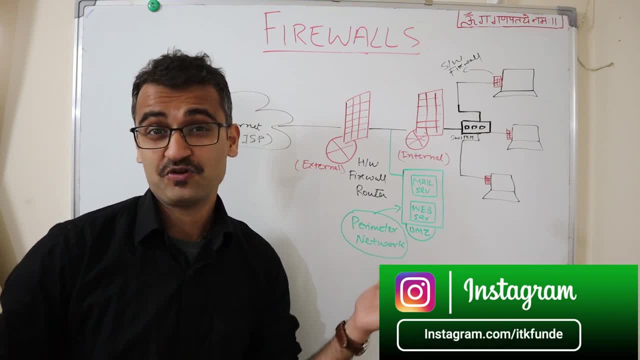 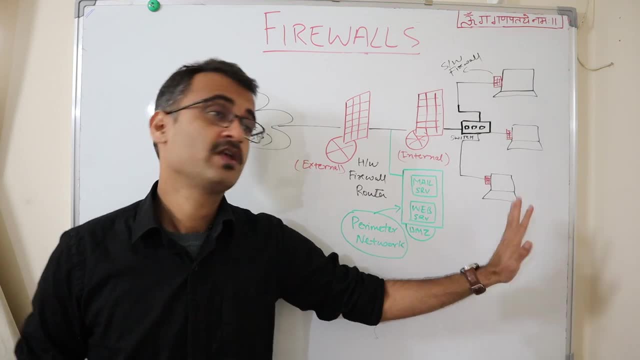 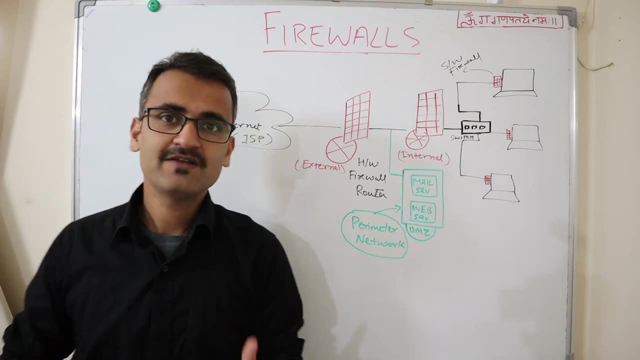 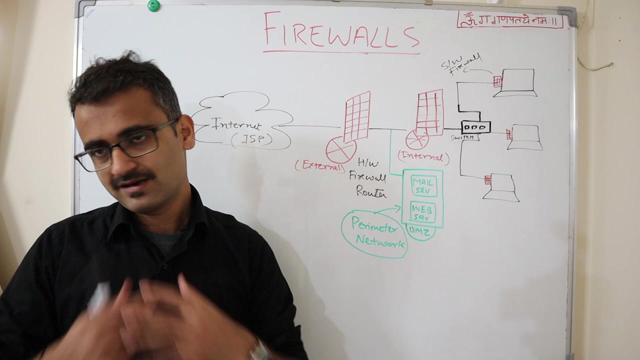 preventative, then the security guard won't ask that many questions, or maybe none. no, no questions would be asked from that particular owner, right, because he has the higher authority. so, in the similar way, when you design your firewall rules, these are designed in this manner. now what we'll understand? we'll understand some basic, broader categories and types of firewalls which we have, the category you know. these are ever expanding and we have new technologies coming up. but these are some basic types of firewalls which you should be able to use and we will discuss more about this later. 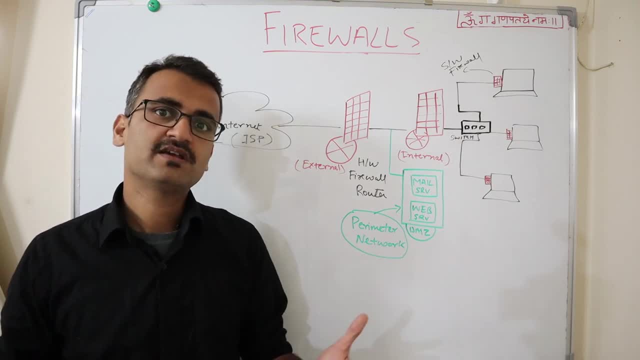 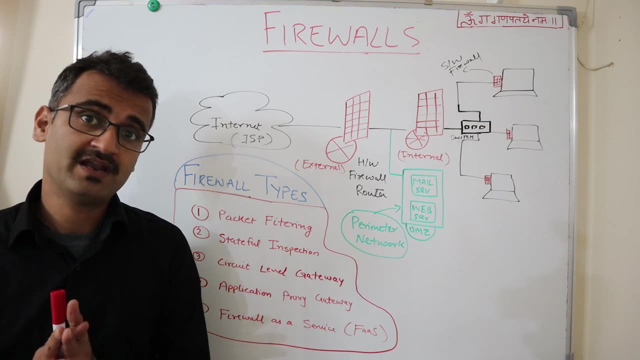 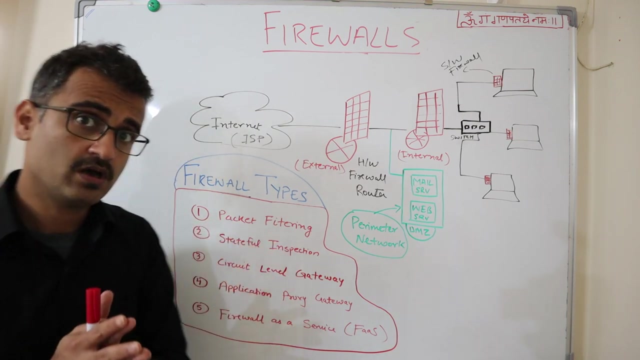 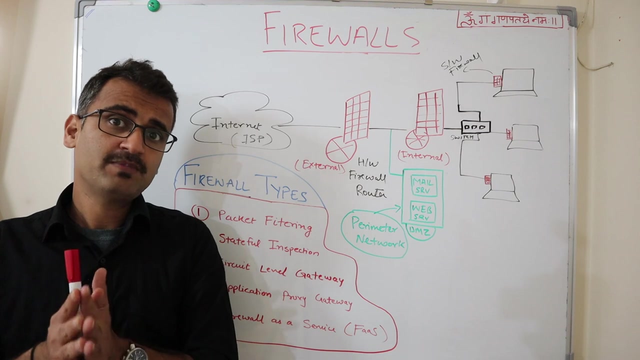 bye aware of. So, friends, now let's understand the five basic types of firewalls which we use in networking. So the most basic type of firewall is packet filtering firewall. It is the most basic but one of the most widely used and efficient firewall type. It inspects any 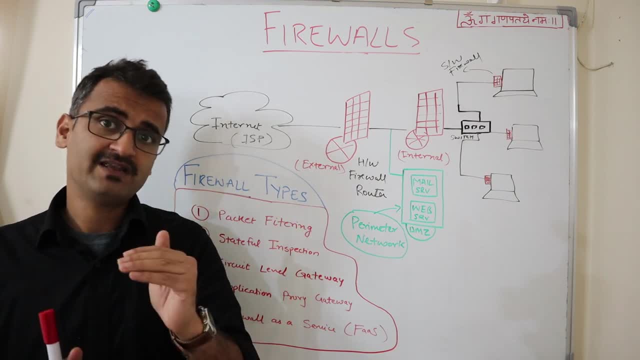 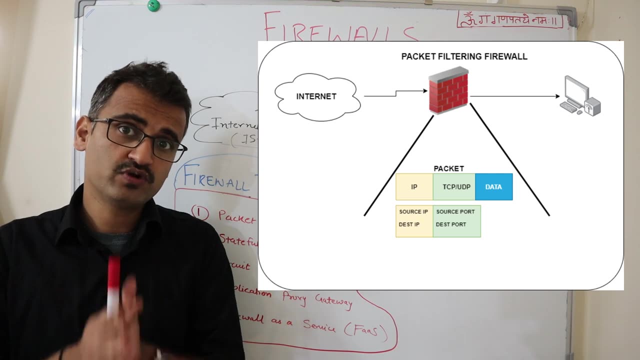 particular network traffic at a very specific packet level. So it would check the source and the destination IP addresses and the port information And based on that it would decide and based on the rules which are given to that particular firewall, it will decide whether this 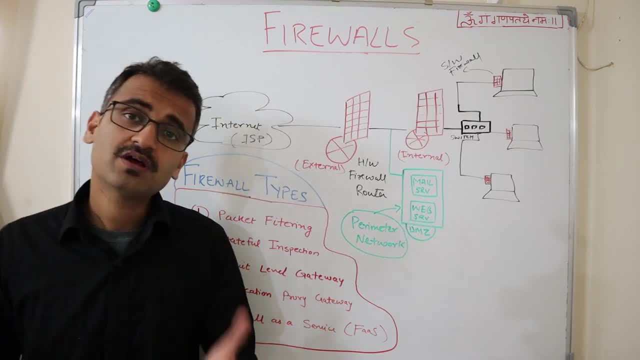 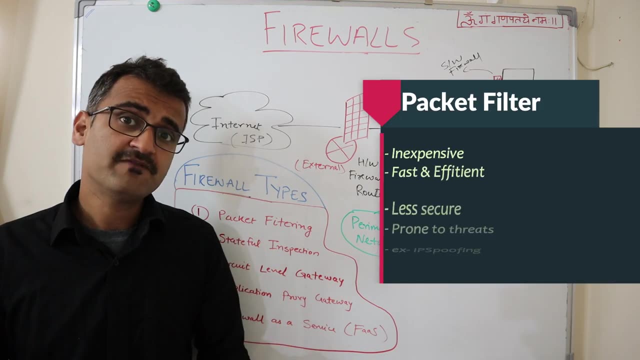 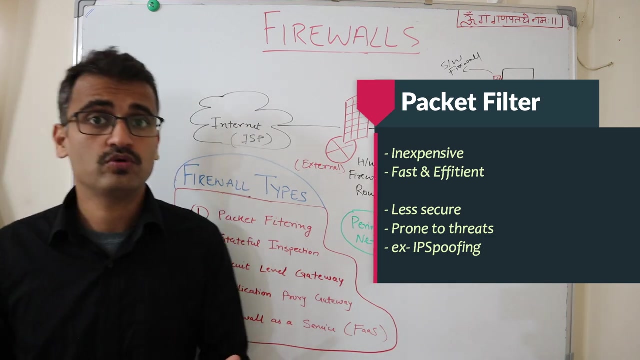 packet is a legitimate packet or not. So what are the good things about packet filtering? The packet filtering firewall is very inexpensive. It's very cheap. Secondly, it is very efficient because it is only inspecting at a packet level. But the downside is that it is not that secure You can. 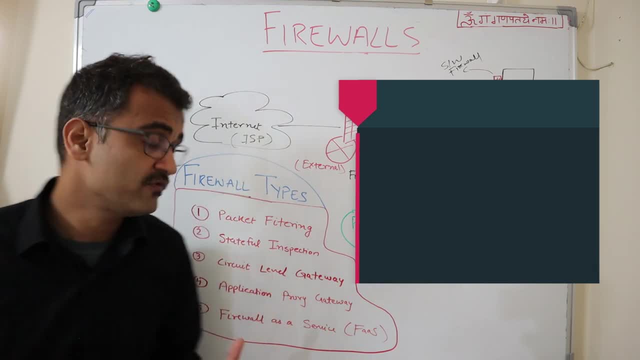 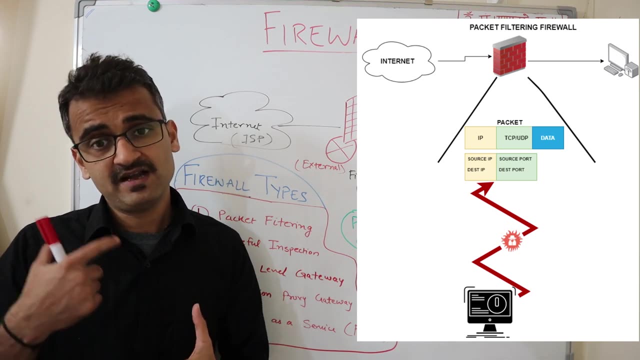 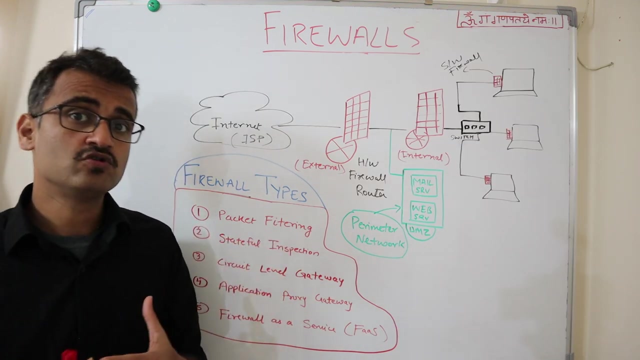 have some attacks Like IP spoofing. And now what is IP spoofing? IP spoofing is if someone injects a wrong IP within that particular packet or forge the IP address And you know it can trick this particular firewall using IP spoofing kind of methods. That's why packet filtering is not considered as the most. 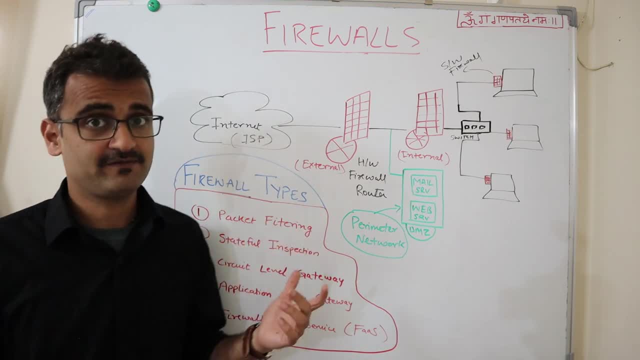 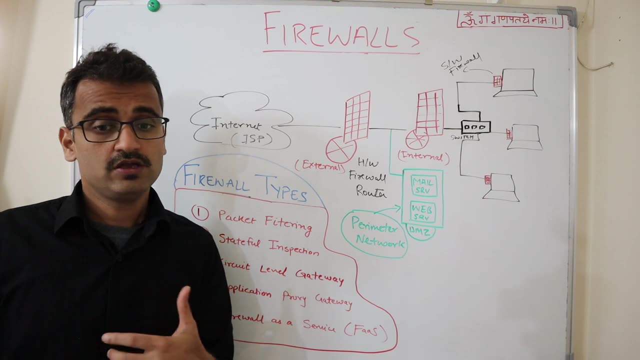 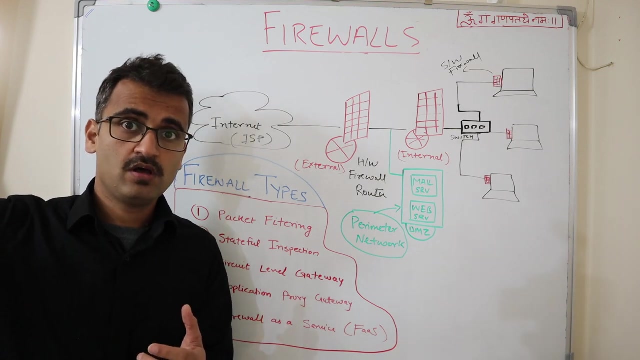 secure, but still it is very widely used because it's very effective. So packet filtering- if we correlate it with our society example, it's as if you know any visitor is coming to the gate and only telling that he wants to visit a particular house. This is the flat number. This 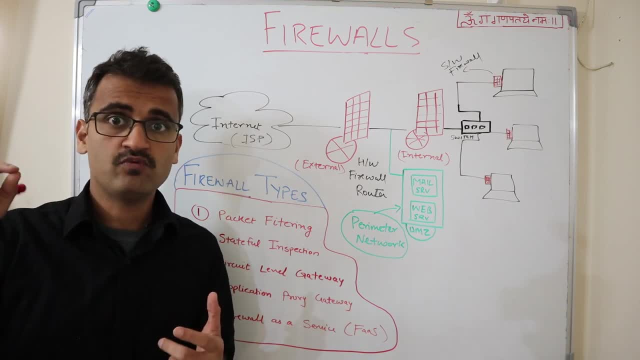 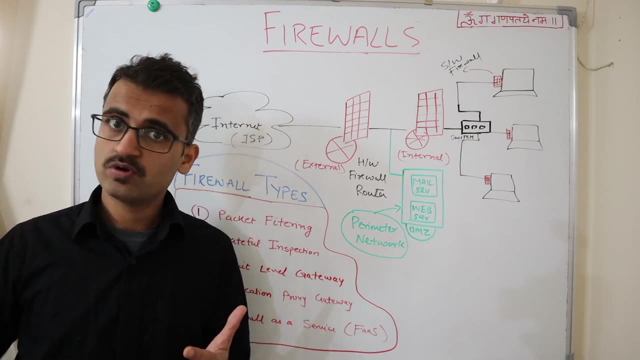 is the owner name and he wants to meet And the security guard only checks that. okay, yes, this is the flat number and here this particular owner stays and he just lets this particular visitor go in. But what if this particular visitor is forging? you know this identity of his and there 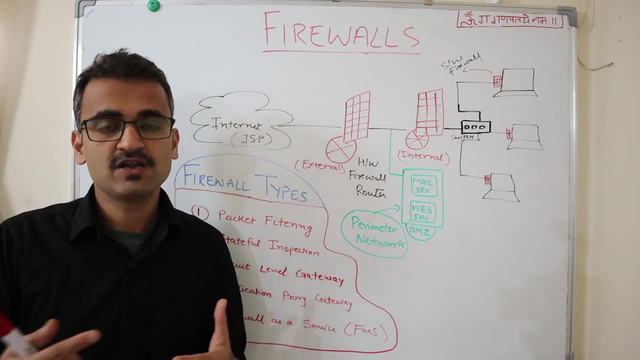 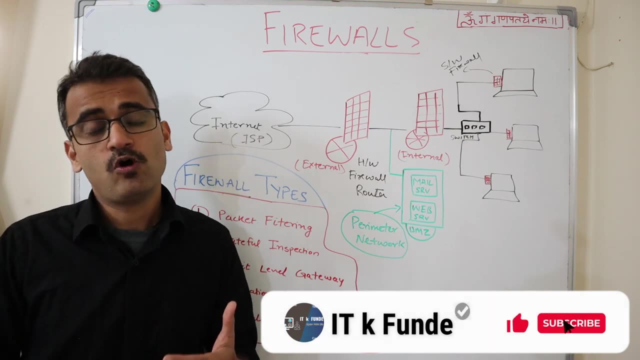 is no inspection, So packet filtering is not considered as the most secure, but still it is very effective. Okay, So packet filtering is the most secure method. The second type of, I think the思 nog. this is also very effective. This is like the most effective way toOr, if you 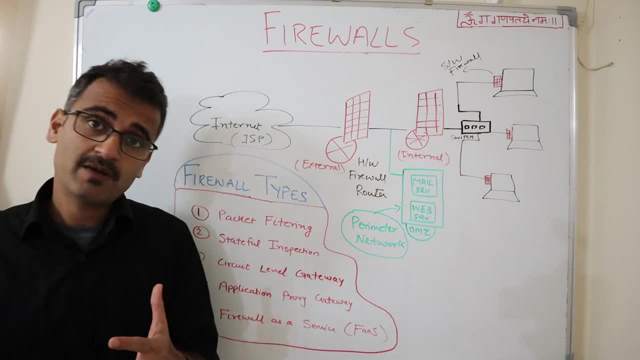 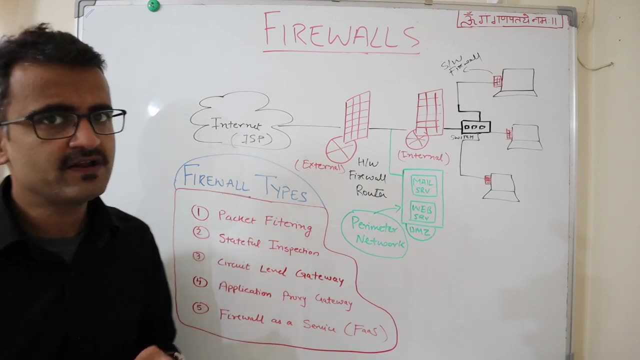 want to validate a particular site, for example. for example, when you want to mail an order from RSS, you can just send an email to the officer and the officer can send that email and get a type of packet filtering. And then the second type is the stateful inspection. 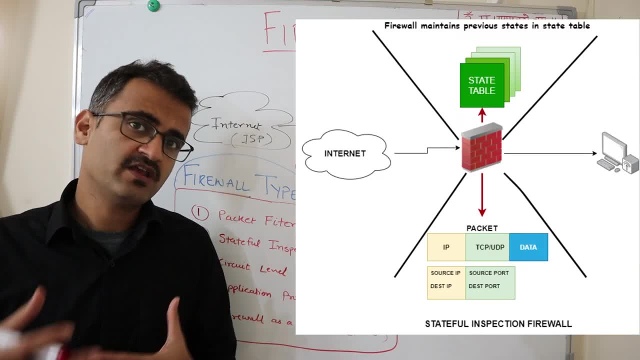 Okay, So then we will start with stateful inspection, and really the easiest thing to do is to inspect packet filtering. Tja now, stateful inspection is an intelligent version of packet filtering traffic which is coming in, so it is keeping a track of previous packets, which. 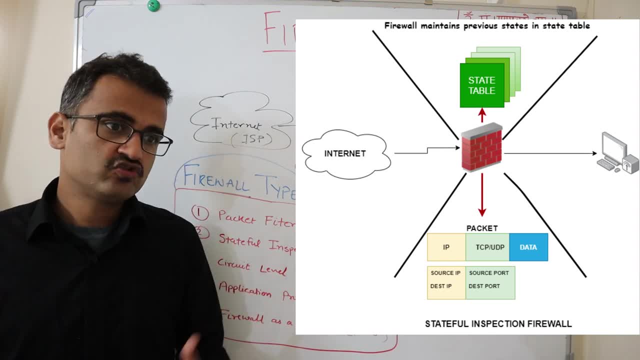 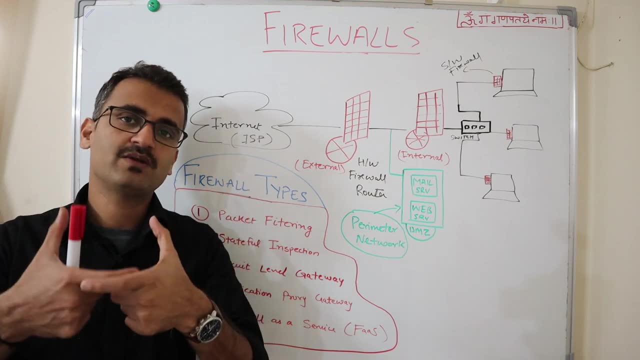 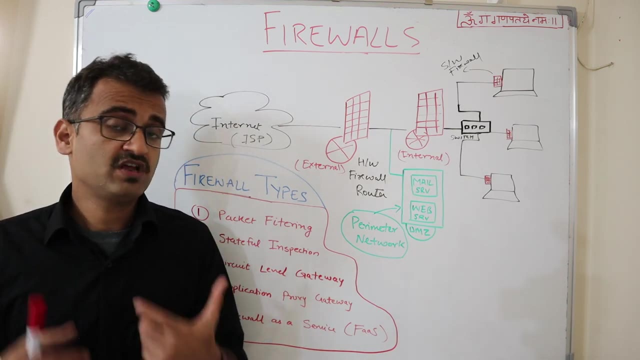 has gone in and the new packet which is coming in. so it would give the additional layer, layer of security, because it's not just blindly taking one packet at one time and allowing it. so take, for example, if any visitor is coming into the society, that guard is not just randomly letting this. 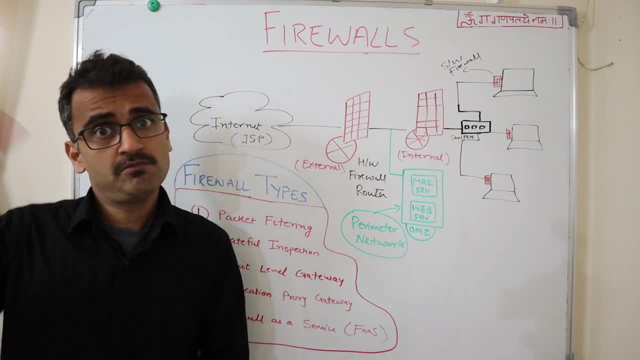 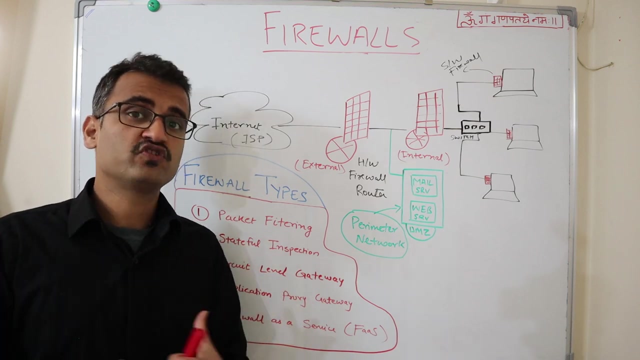 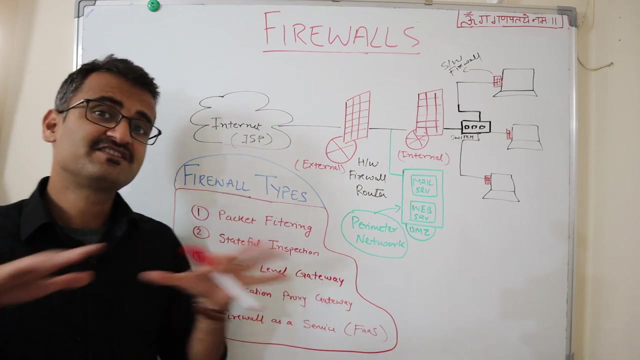 particular visitor go in. it is validating. maybe you know calling the owner, checking whether you know this particular visitor was called for, you might understand what is your objective of coming in. take more detail, something like that. so adding more context would give more security. adding more context to it gives you a stateful inspection. so this packet filtering is stateless. you're. 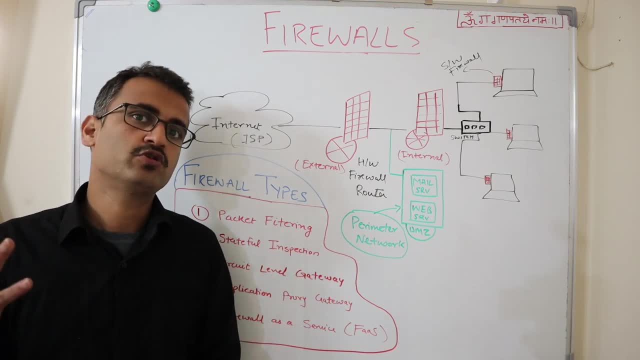 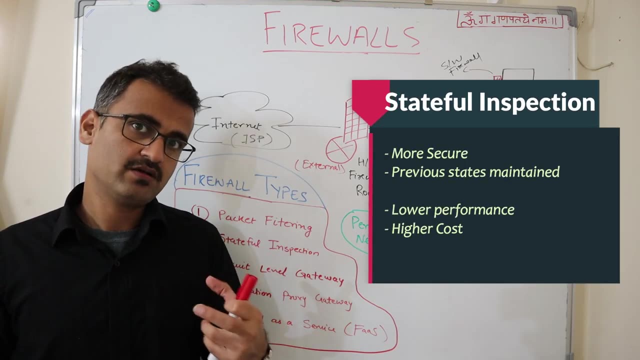 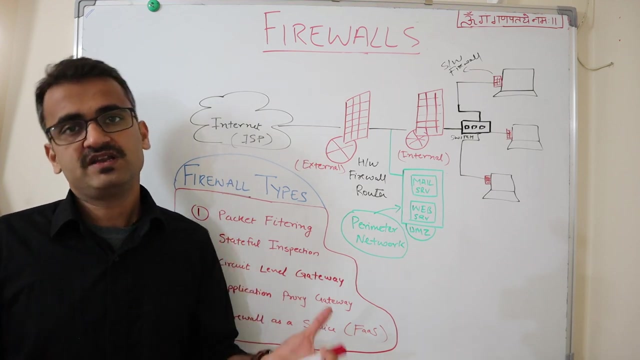 not worried about the state. you are taking one packet at a time and you are taking a call here in, whereas in stateful. you are understanding the context. so it is slightly higher. you know secured version, but obviously it comes with a cost. it would be slightly expensive, it would be slightly slower, but yeah, it all boils. 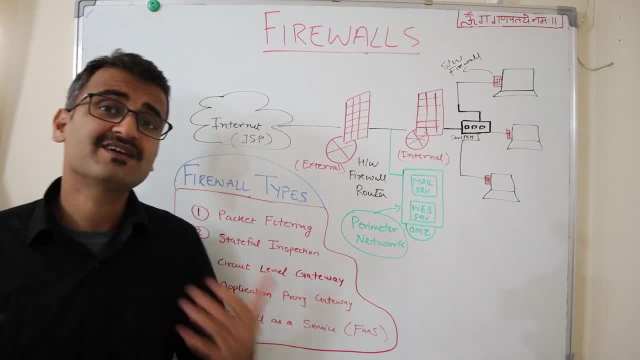 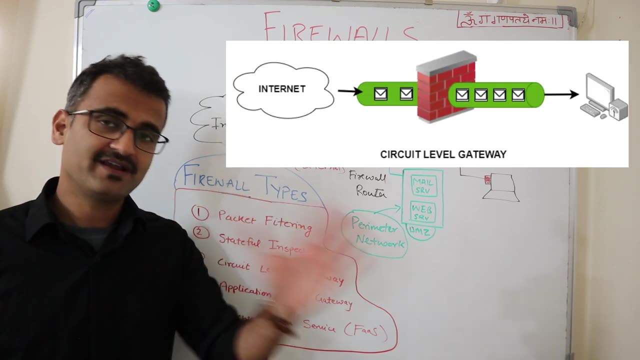 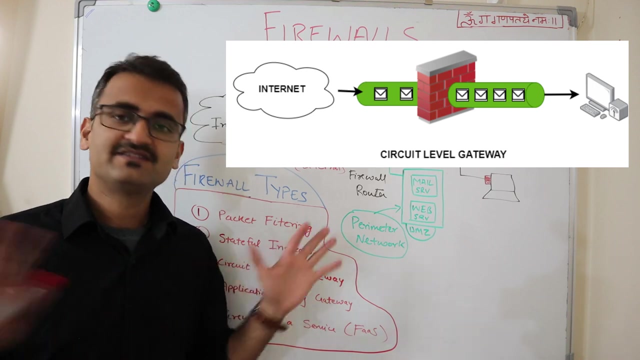 down to your requirements. the third one is circuit level gateway. now, in circuit level gateway, the firewall establishes, you know, a circuit, a tunnel of sorts, between source and the destination. it connects both the network at once, and then it just goes out. the firewall says: I have now. 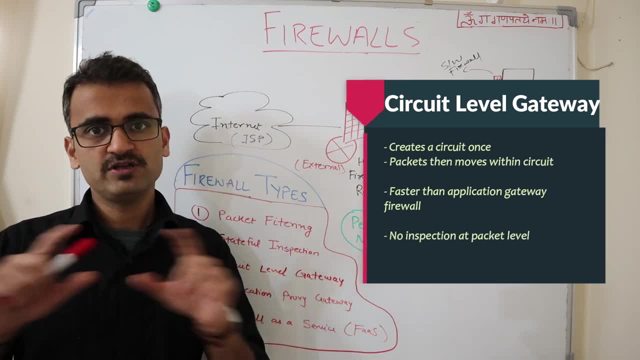 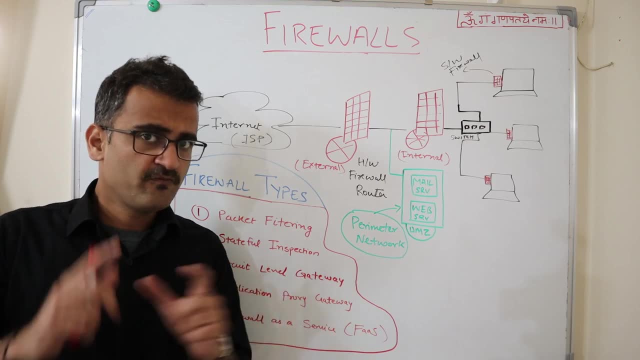 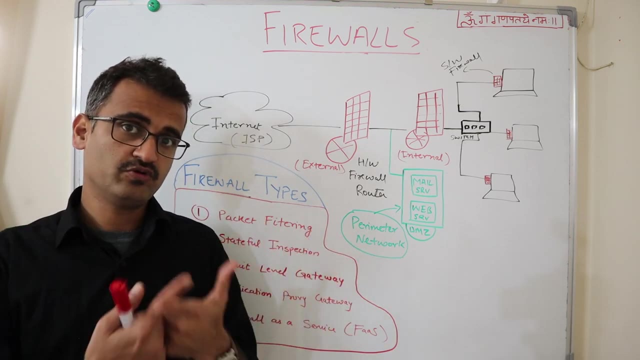 connected you, I have validated. I have connected you through this particular port. now do whatever communication you want to do. the firewall won't interfere in that. so VPN is kind of you can understand a similar concept where you create a VPN tunnel and then you continue to interact. so suppose, if you 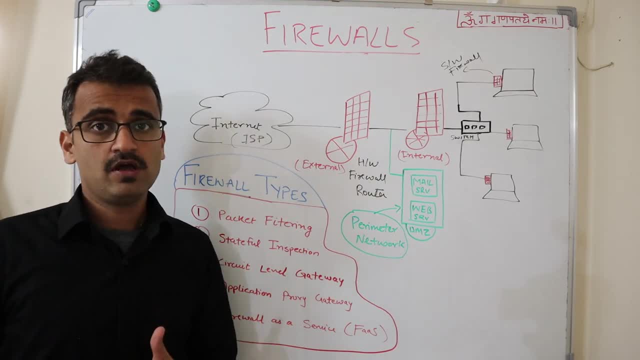 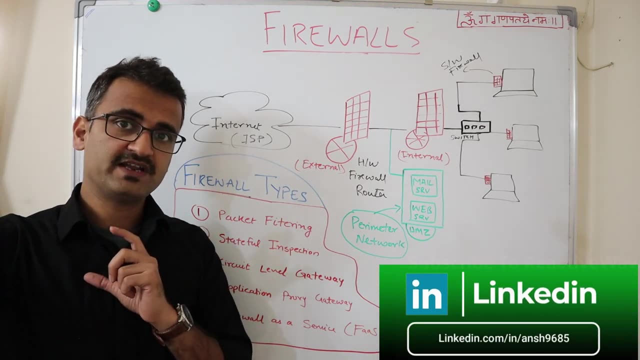 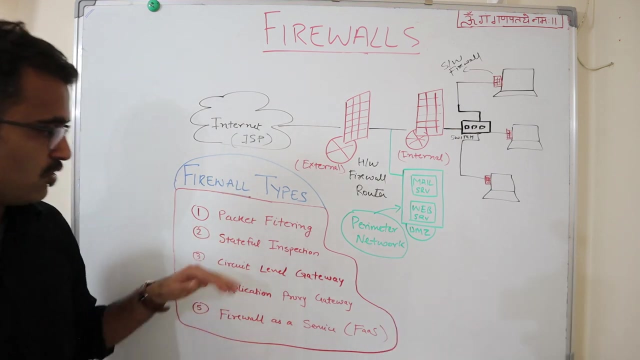 are doing a talent from your client machine to a server and if there is a circuit level gateway in there, so the moment you connect to your telnet port, that particular tenant channel would be created and then the firewall would- just, you know, won't interfere in the further communication. now, again, again it has. 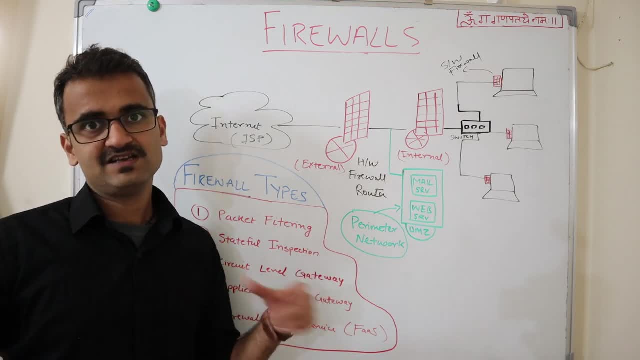 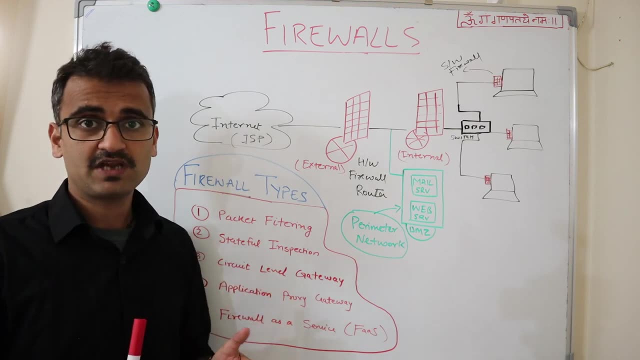 some goods and the bad, so good is. once it is there, the channel is created, it's very seamless. but again, what happens, if you know, if something goes wrong? because now the firewall is not at all taking care of this circuit, it might happen that some kind of interference might happen in this. 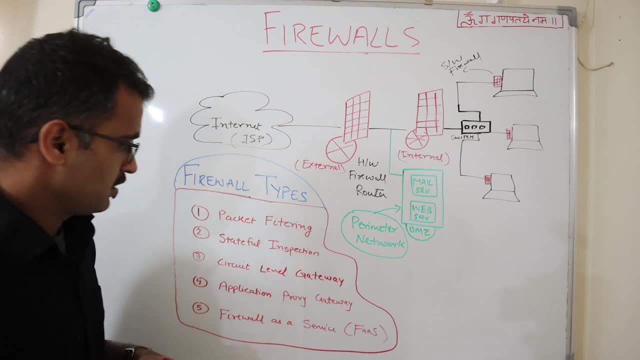 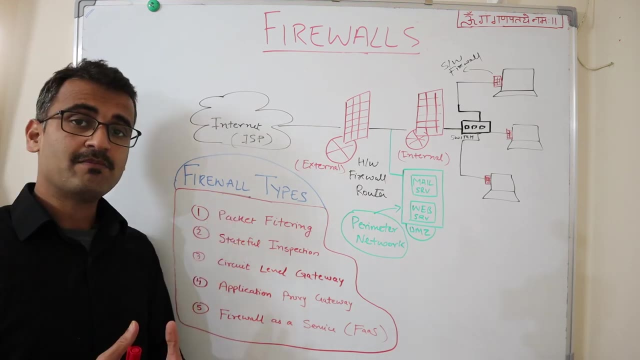 so the thing that you have to be careful about is that you need to have a. so, again, this has some drawbacks. now application proxy gateway. this is the by far the most superior version. it combines all the goods of the top three and then offers something more. so now application. 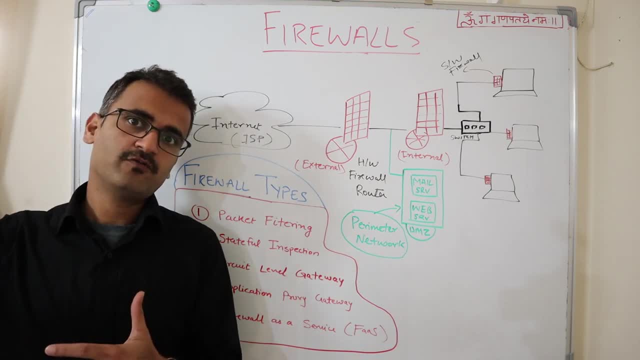 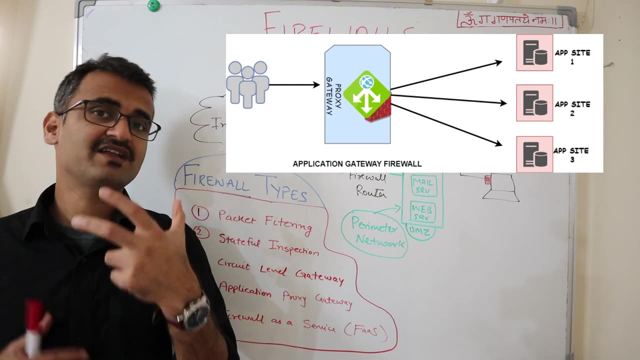 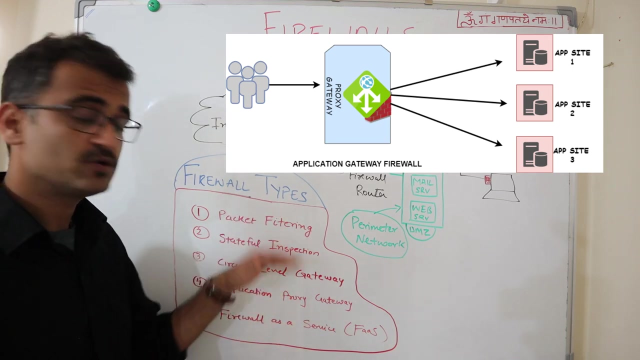 proxy gateway works at a, you know, higher level of osi model. so it it works at an application layer and what it does is it takes the application context into picture and then deploys the firewall rule. so the firewall is way far intelligent compared to this. because these are 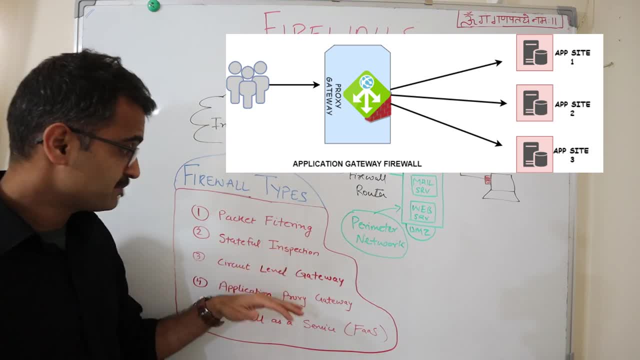 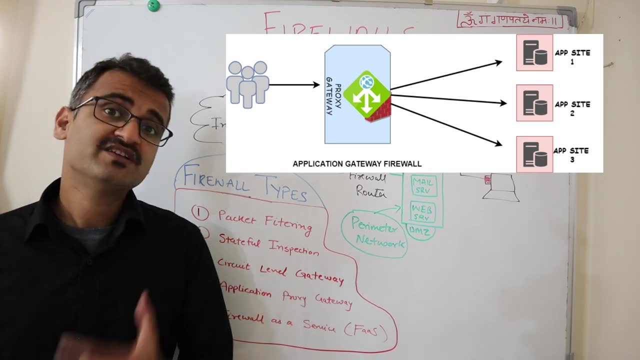 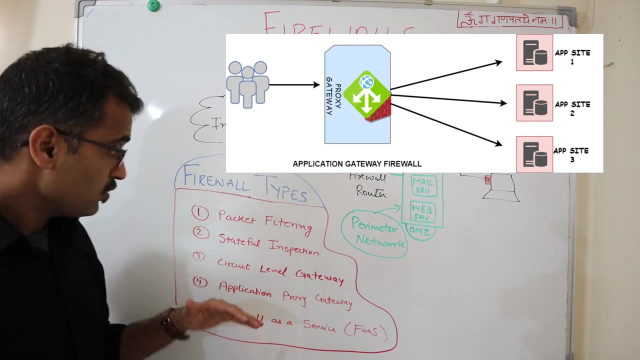 uh, basically working at a network layer or a transport layer. this particular proxy gateway is dedicatedly working at an application layer, so it it knows what this particular application is expecting. so suppose there is a web application which is expecting some site, sort of an http traffic, to come in. now this particular firewall could be deployed with an. 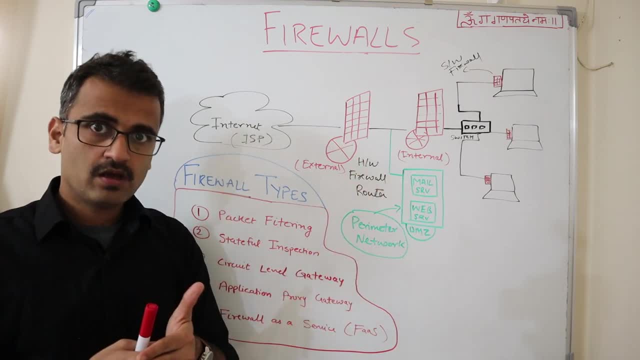 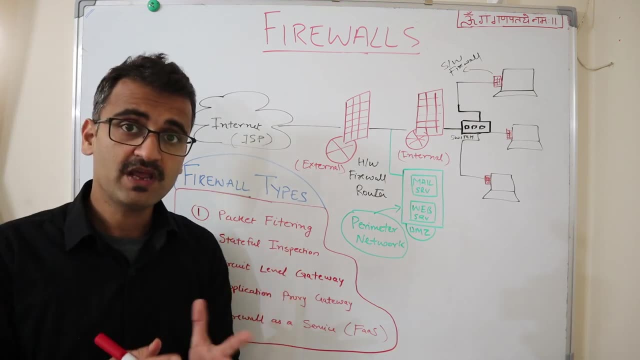 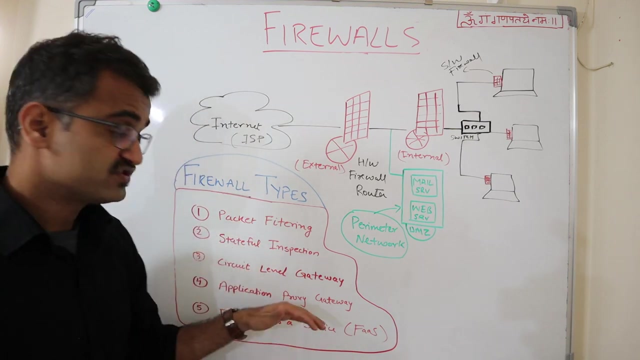 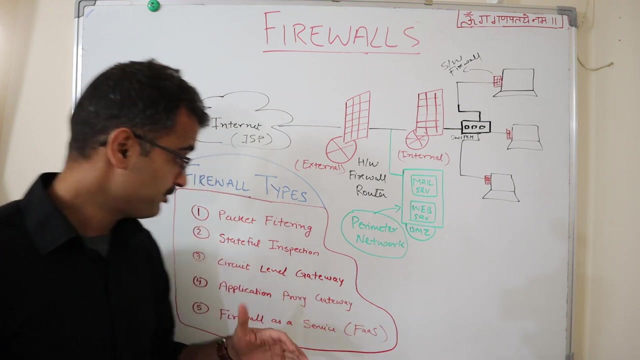 intelligence to assess the packets which are coming are actually in the design format or not, and it might see that, okay, this particular http format which is coming is not correct. it might redesign it to the in a manner in which the application is requesting. also, suppose there is certain pages of this web application which are static, so those can be cached at a this. 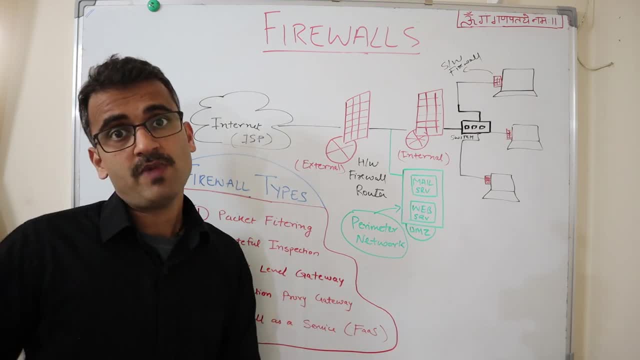 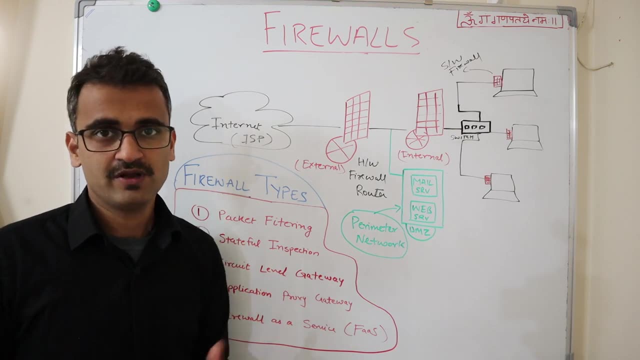 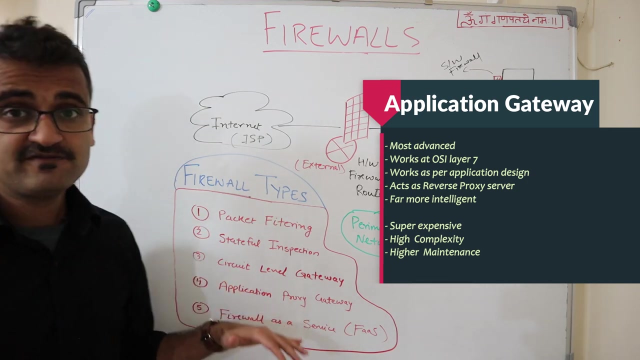 particular gateway level so the request might not again go back and come. for these kind of static pages it, this particular firewall gateway could manage this on its own. so this is by far the more most intelligent version of all the four which we have talked about, but very expensive and takes a lot of. 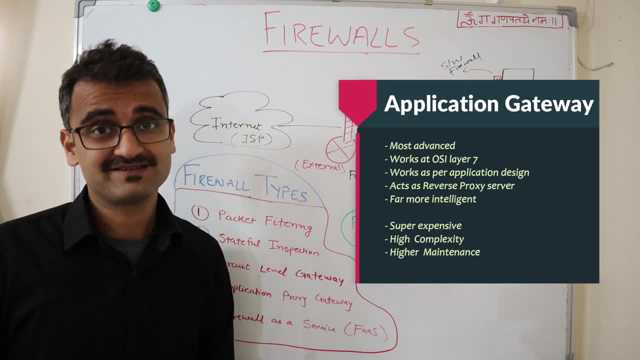 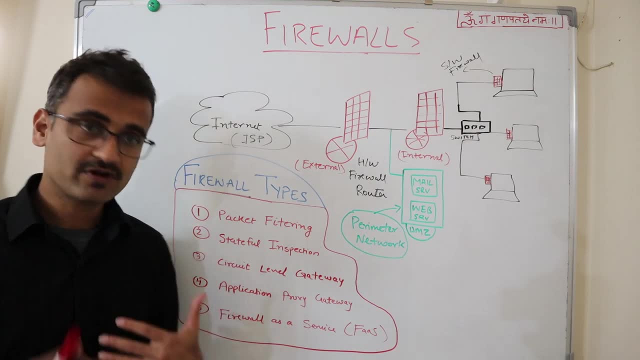 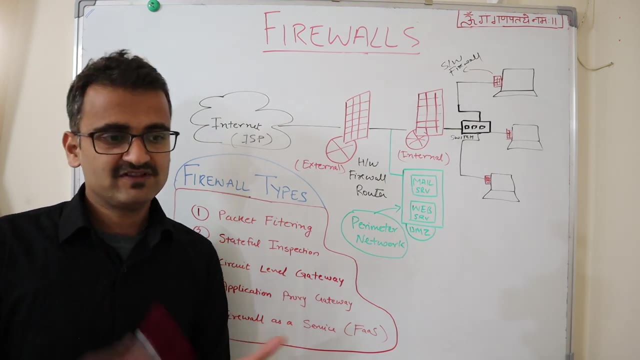 maintenance and designing these kind of firewalls are way more complex technically. and last but definitely not the least, is firewall as a service. now, what is firewall as a service? you you might know that now more and more applications are going on to the cloud and you have these big 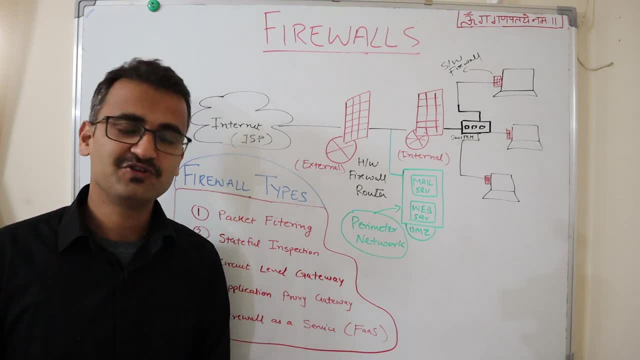 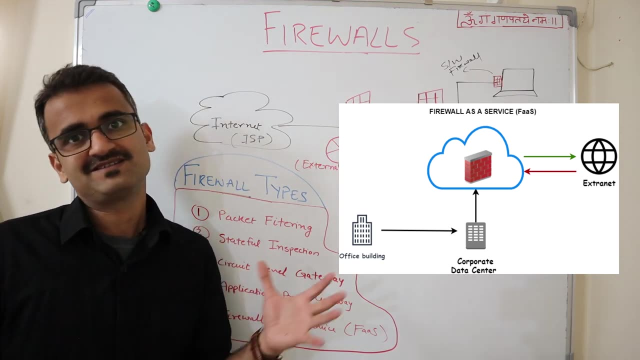 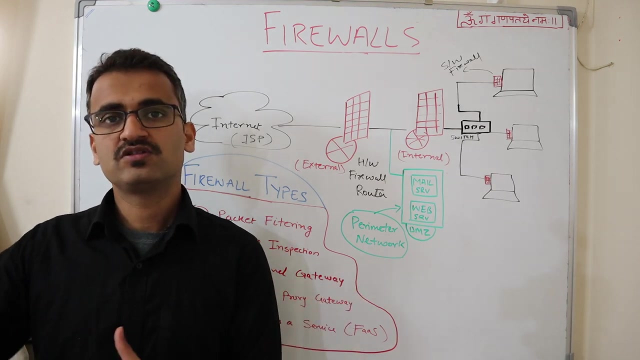 cloud providers who are offering you firewall as a service. so you take, for example, if we talk about google cloud platform. so in google cloud platform you can design your whole firewall just from the web portal or the gui of cloud vendors and you don't have to worry about the internal. 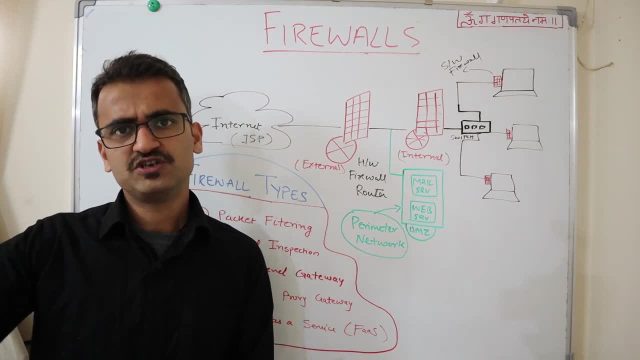 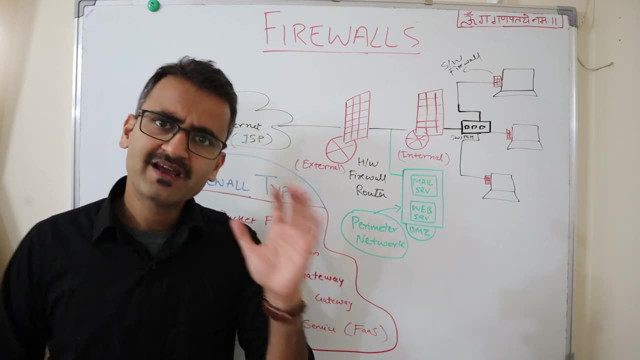 functioning of it. you just need to decide, okay, what kind of rules you want. you just go there and you just select whatever rules- inbound rules or outbound rules- you want, and rest. all will be taken care under the hood by the cloud provider. so this is now very, very much emerging, which is